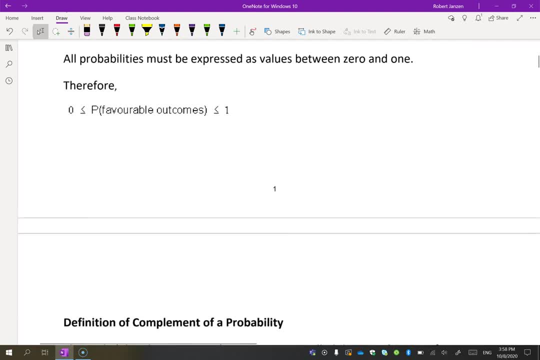 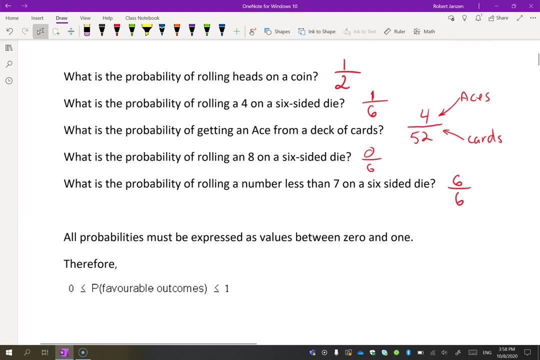 So let's try a few questions. Sorry, not quite. We're not quite done here. All probabilities must be expressed as the values between zero and one. So if you look at all of these numbers here, okay, what's the biggest number that you have? The biggest number would be six out of six, which is one. 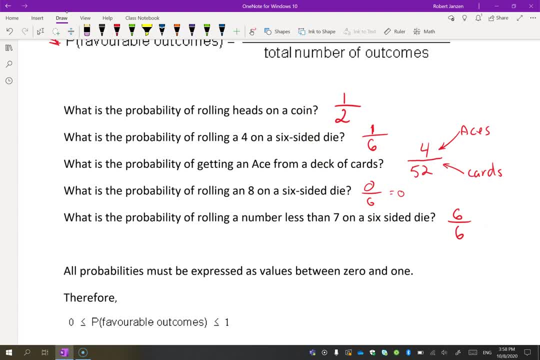 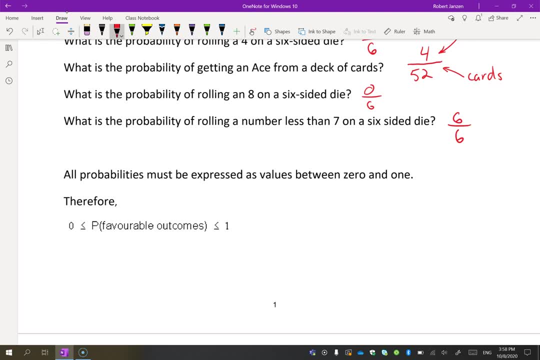 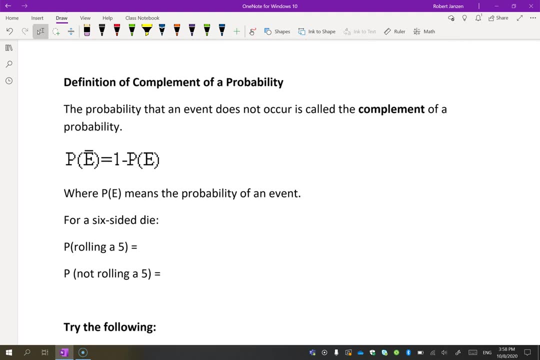 The smallest one would be zero. Probability can't be less than zero and it can't be greater than one, So it's always going to be something between zero and one. That's what this means. Okay, And then we have something called the complement of a probability. 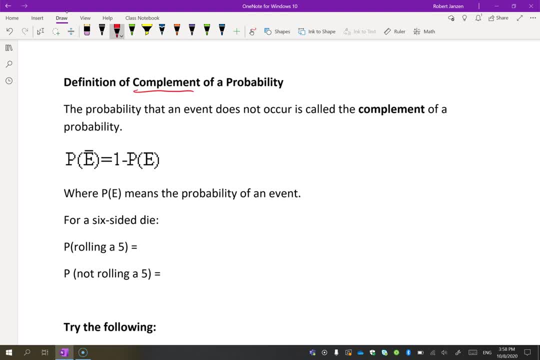 The probability that an event does not occur is the complement. Okay, So let's look at an example For a six-sided eye, the probability of rolling a 5, that's 1 out of of 6.. The probability of not rolling a 5,. 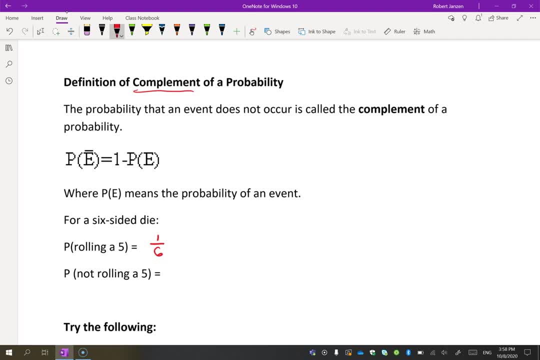 well, you can already see that's 5 out of 6, but looking at our formula here, the probability of not rolling a 5 would be one. take away the probability of rolling a 5, so 1. take away 1 over 6,. 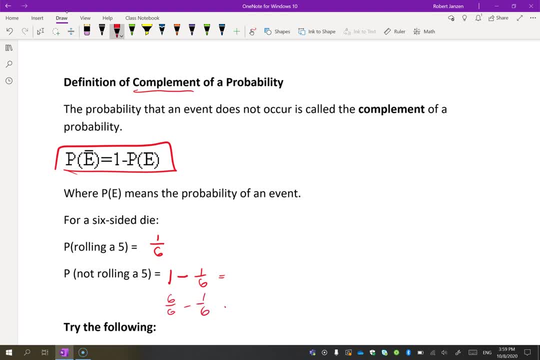 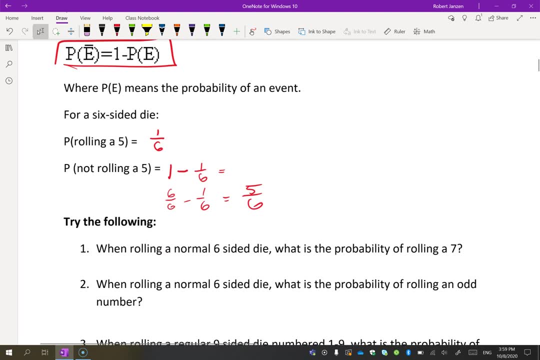 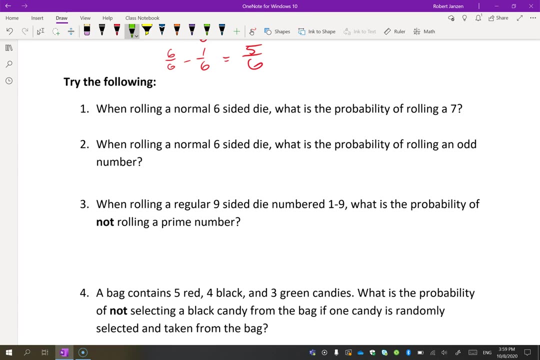 which, if we do the math, the math here, this is six over six. take away one over six, you end up with five over six. okay, so that's what the complement is. it's the opposite, sort of the opposite of something happening. okay, a few questions here. when rolling a normal six-sided die, what is the probability of rolling? 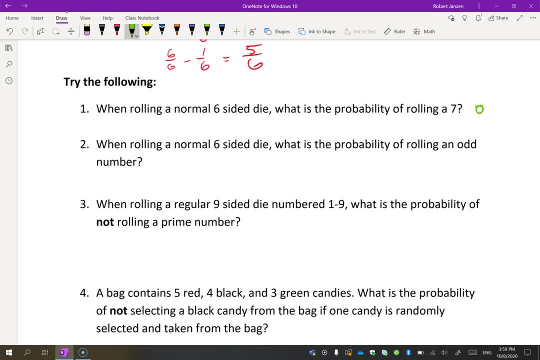 a seven. well, we already know there are zero possibilities: not out of seven, out of six. okay, when rolling a normal six-sided eye, what is the probability of rolling an odd number? well, the numbers that are odd are one, three and five. so that's three favorable outcomes out of six. 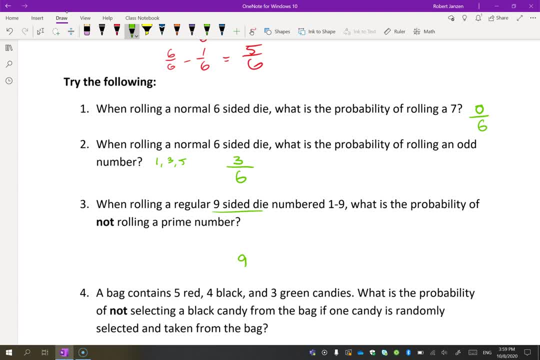 okay when rolling a nine-sided die. so there are nine possibilities. what is the probability of not rolling a prime number okay? well, first of all, we need to know what a prime number is. a prime number is any number of a die that is not out of six. 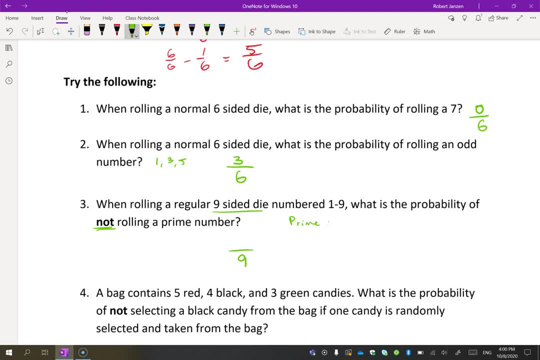 number that can be divisible by one and itself. so two is prime, three is prime, five is prime, seven is prime. all of the other numbers between one and nine, like one, only has one factor and all the other ones have more than two. okay, the prime number only has two factors. so this is the probability of a prime number. 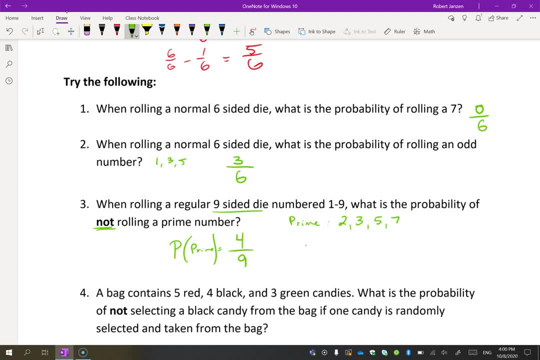 would be four out of nine. so what's the probability? i'm gonna write it in a different way here: what is the probability of not a prime? so this is one takeaway: four out of nine, which is five out of nine, okay. a bag contains five red, four black, three green candies. 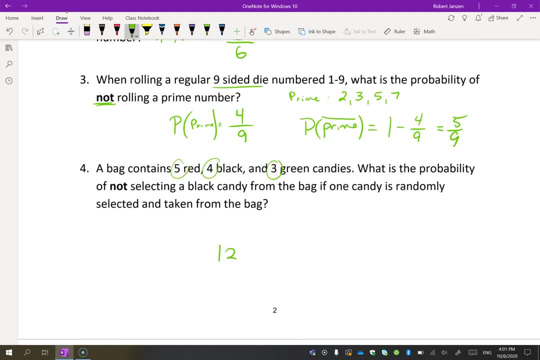 if you add those up, there are twelve possibilities. what is the probability of not selecting? selecting a black candy, Okay, so what is the first of all we should say? what is the probability of black? So what is the probability of not selecting a black candy from the bag? 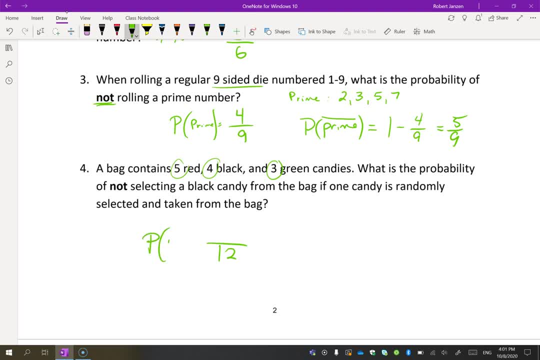 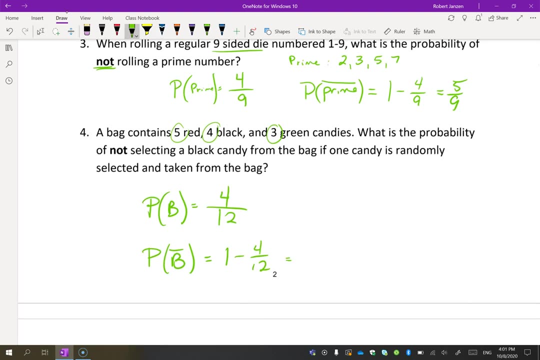 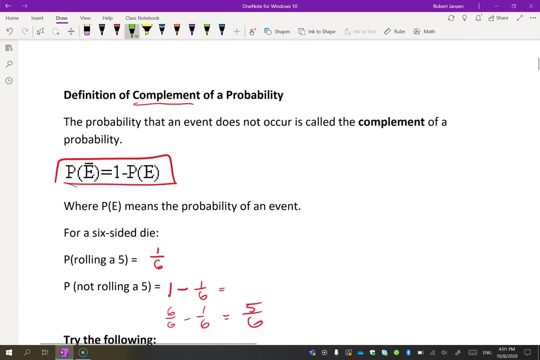 if one candy is randomly selected. So what is the probability of black? It's 4 out of 12.. So what's the probability of not black? Well, this would be one takeaway: 4 out of 12.. Okay, and that's 8 out of 12.. Okay, now just going back here a little bit, this is: 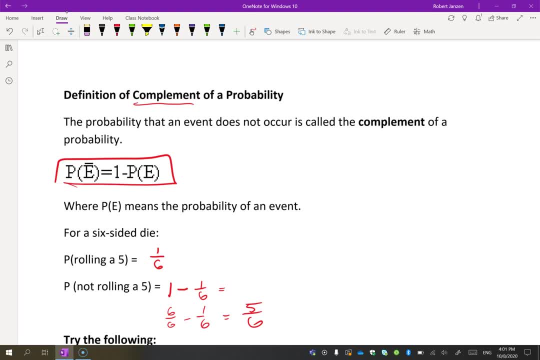 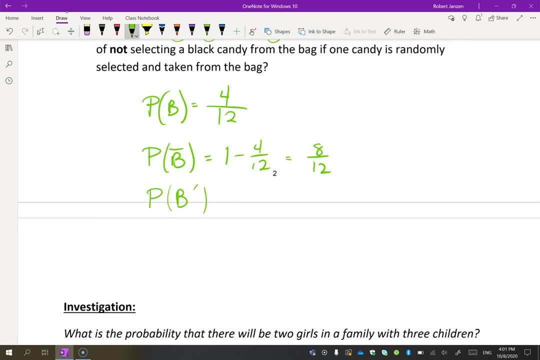 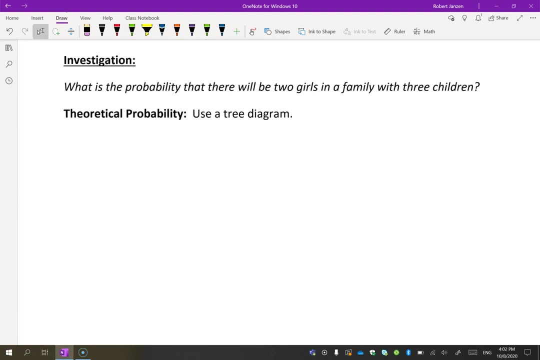 one way of writing, not something We have that solid line over. I've also seen it with B prime like that. Okay, either of those is fine. Okay, what is the probability that there will be two girls in a family, A family with three children? Use a tree diagram. Okay, so, first child, second child, third. 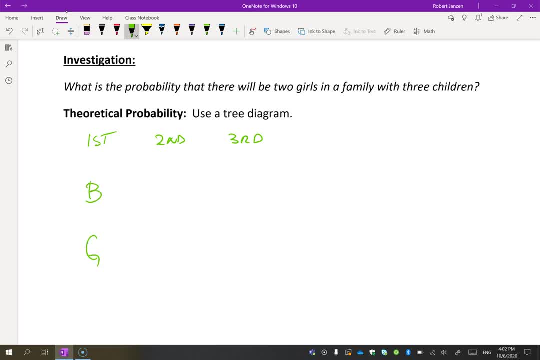 child. So the first child could be a boy or a girl, Second child could be a boy or a girl, And the third child could be a boy or a girl. Okay, so listing all of the possibilities here, we have boy, boy, boy. We have boy. 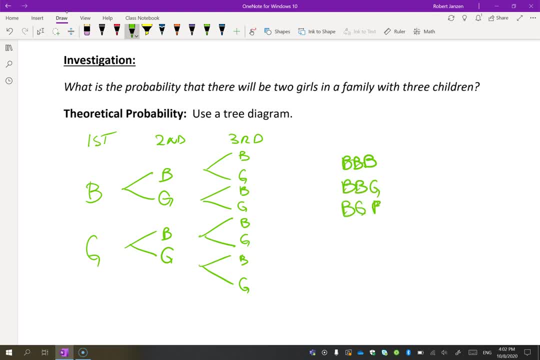 boy, girl Boy, girl boy, Boy, girl girl. So I'm just following these, Okay, and then the next one would be girl boy boy, Girl boy, girl, Girl, girl boy And girl girl. 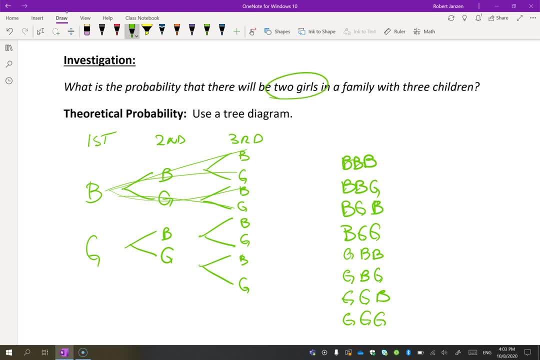 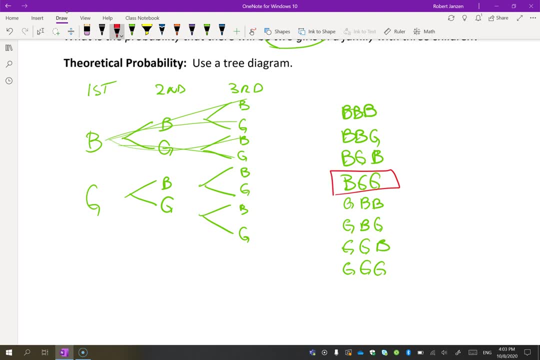 girl 12.. what is the probability that there will be two girls? Okay, so that's two girls, Here's one, here's two, here's three. The probability of two girls is three out of eight. Okay, so now let's get into experimental probability. 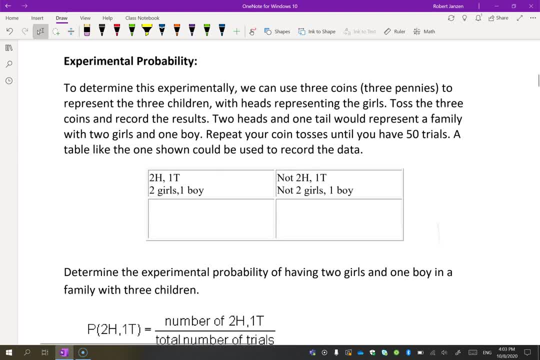 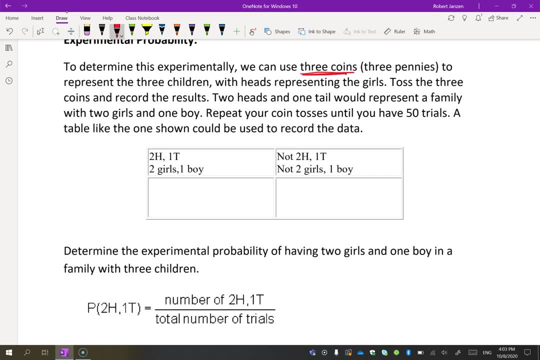 I would like you to try an experiment Now. everybody's going to have different answers here, so the notes are going to be a little tricky, But what you're going to do is use three coins, okay, three pennies, dimes, nickels or whatever. 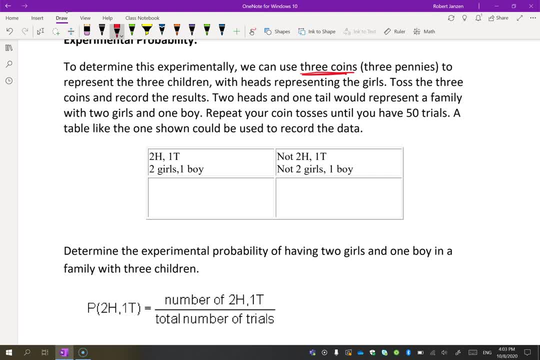 to represent three children with heads representing the girls. So if you you know, here's your three coins. If two turns out head and one turns out tails, this would represent two girls and one boy. Okay, So what you're going to do is toss three coins 50 times and each time you record what you get. 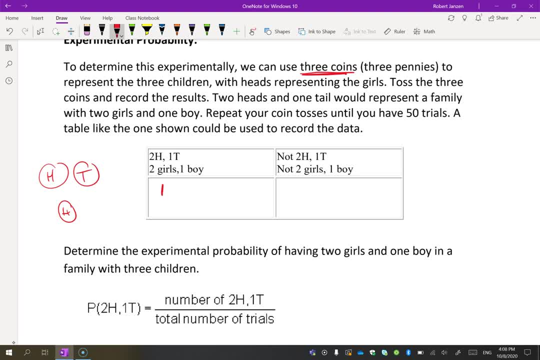 So if you end up with two heads and a tail, you would put a tally mark here. If it's not two heads and a tail, you would put a tally mark here. Okay, and you're going to do this 50 times, whatever you end up getting. I don't know. 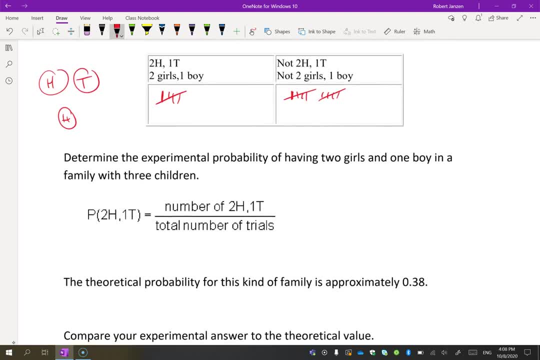 Okay, so go ahead and try that, And once you've done that, you can unpause the video and then come back to this. Okay, so, experimental probability: whatever you had here, that's the number that goes on the top. Whatever you had here, plus if you add these two, okay, this is going to be 50.. 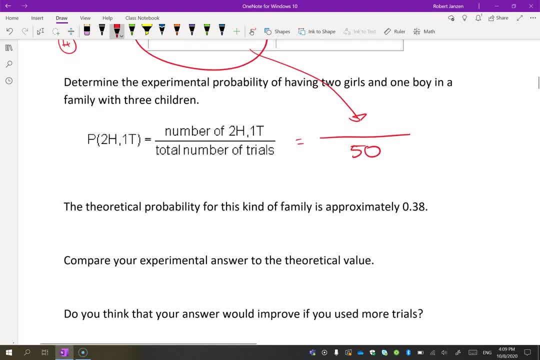 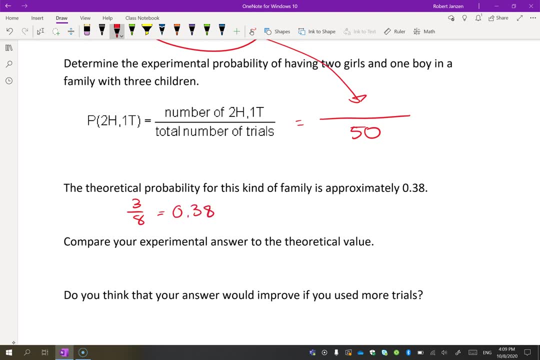 So then we're going to figure out what the experimental probability is. Now we already knew the theoretical probability was 3 out of 8, which is about 0.038.. Okay, compare the experimental answer. So what is your experimental answer? 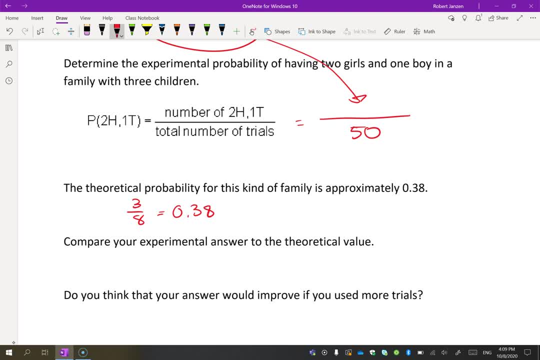 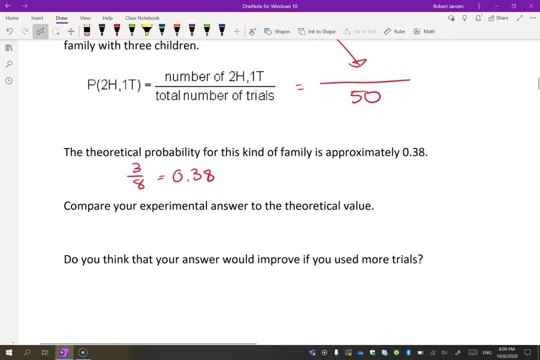 Is it close to this or is it far away? All right, I had expected it would be fairly close, but it doesn't have to be. It could be off a little bit. The point here that we should make is: do you think your answer will get closer to this number when you do more trials? 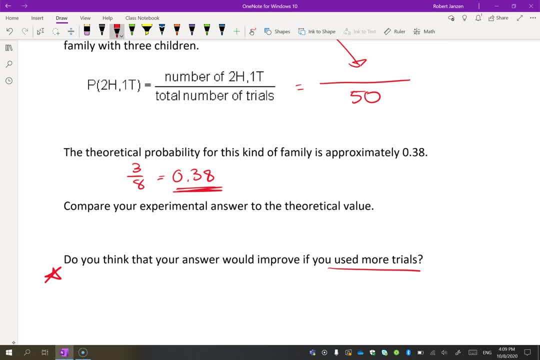 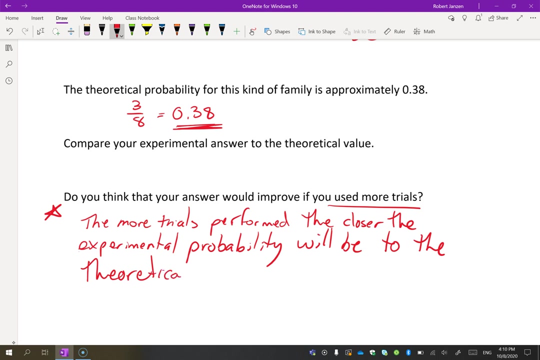 So instead of doing 50, if we did 100 or 200 or 1,000.. So this is the case: The more trials performed, the closer the experimental probability will be to the theoretical probability. Let me go over to my library and do a little more sampling here. 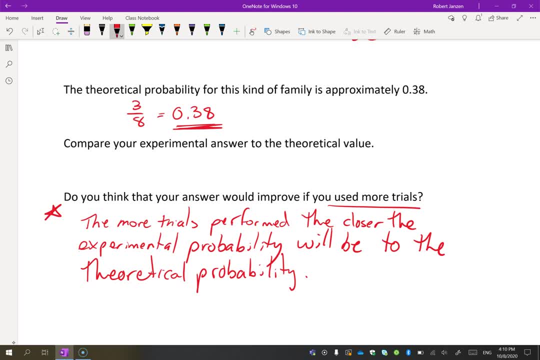 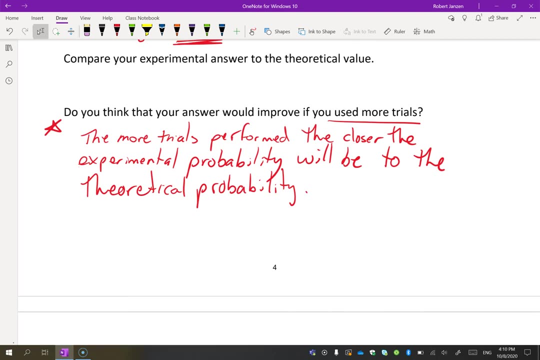 Okay. so what that means is, if we do this trial over and over and over again, then eventually our experimental probability will be very close to what the theoretical probability is. This is a really good lesson to learn. Have you ever played a game where you're rolling a die and you've rolled six in a row? 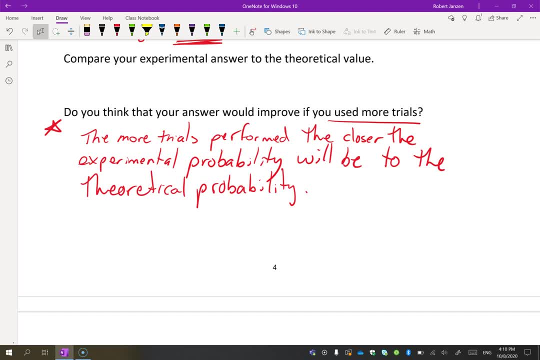 and then the person you're rolling a die on is going to die rolling against might say, well, there's no way you're going to roll six again because you just did it a whole bunch of times. Well, you realize that even if you rolled six, like 10 times in a, 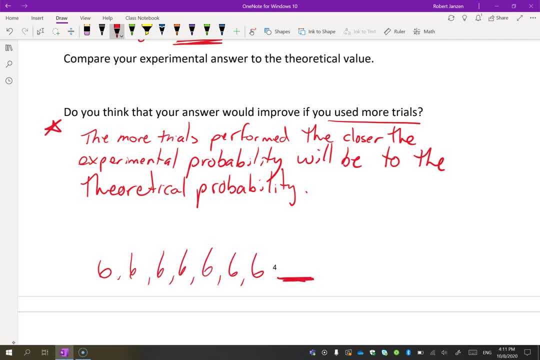 row, which is very unlikely that next roll. what is the chance of rolling a six? Well, just because you've done a whole bunch of sixes does not change this. This is still a one in six chance of rolling a six. Theoretical probability is a better gauge of what the actual probability is Experimental. 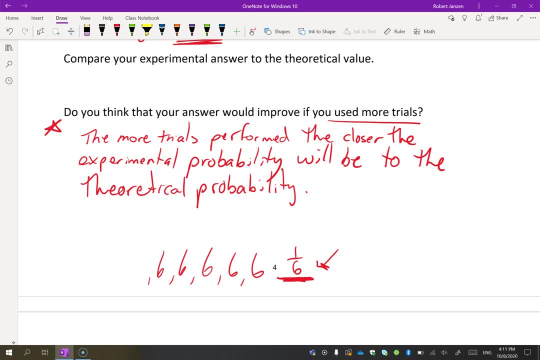 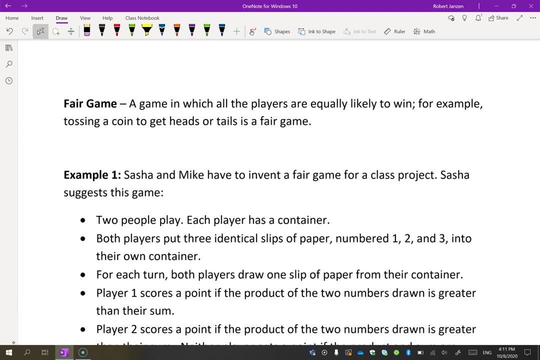 probability is what happens, and sometimes what happens is weird, but the more you do it, the more likely it will be closer to the theoretical Okay, so it's important to keep that in mind. Let's talk about what a fair game is. A fair game is a game in which all the players have an 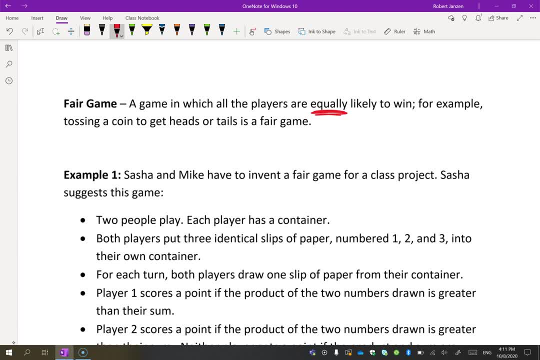 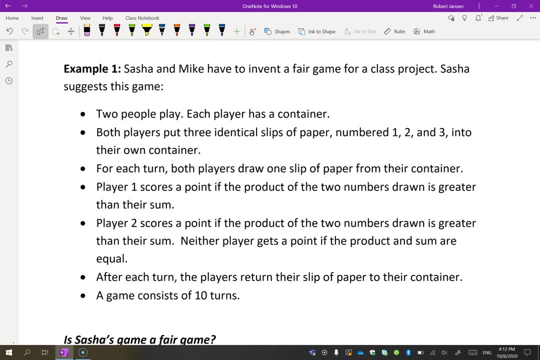 equal chance to win. Okay, for example, if we both have a coin and if you get a tail and I call heads, then we have a 50-50 chance of winning. We both have an equal chance of winning. Okay, so let's take a look at this game. I want. 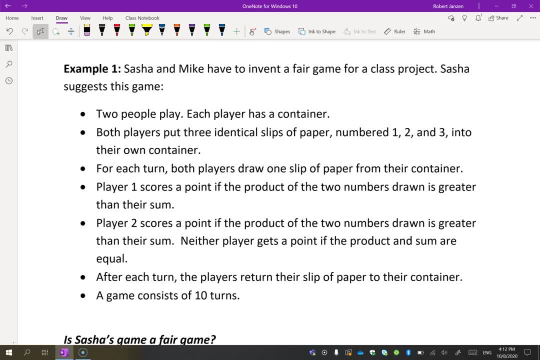 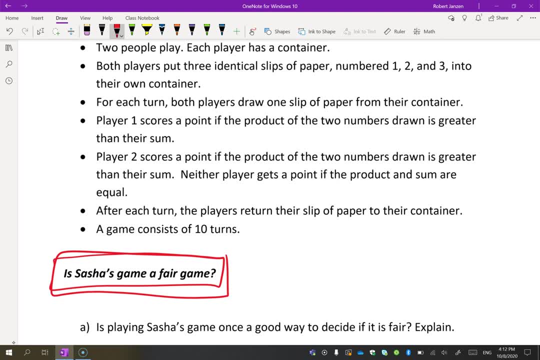 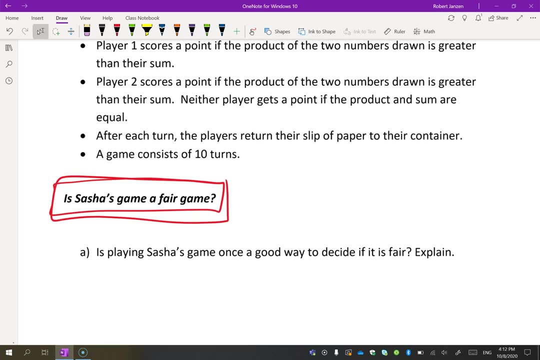 you to take a look at the game, read through this and decide: is the game fair? Okay, so pause the video, read through it, decide: is the game fair, Okay. so you're back and hopefully you've decided. First of all, if I just play the game, 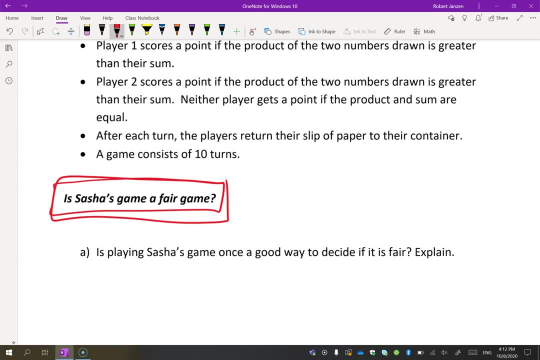 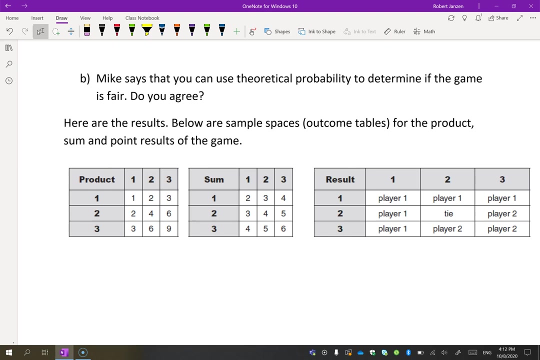 once. is that a good way to decide if it's fair? No, it's not. Okay. the best way to determine if it's fair is to use theoretical probability. In other words, what should happen if we do this? Okay, well, let's take a look at what should happen. Here are the results. So this is what. 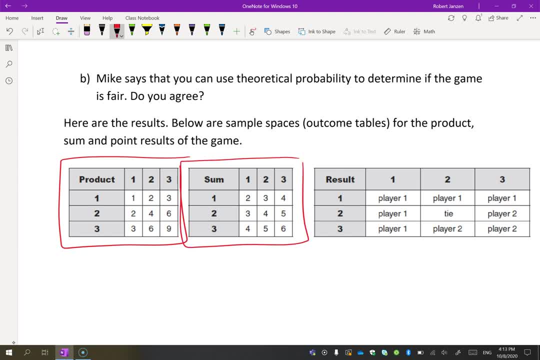 if you take two coins or, sorry, if you take those pieces of paper. all right, these are the possibilities. We could pull out a one and a one. so we could pull out a one and a one, and the product would be one and a one. So we could pull out a one and a one, and the product would be one. 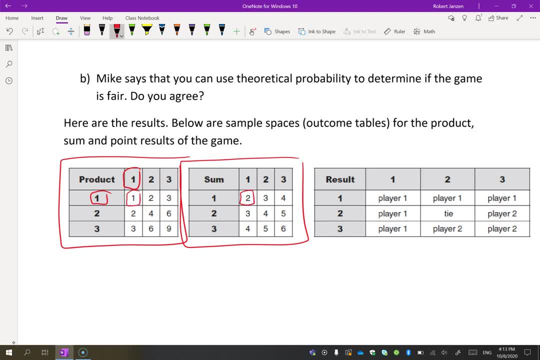 and a one and the sum would be two. Okay, and these are all the possible things that could happen. All right, and you can see that. what? if both numbers are ones, player one wins. If we have a one and a two, player one wins. If we have a one and a three, player one wins. These two places. 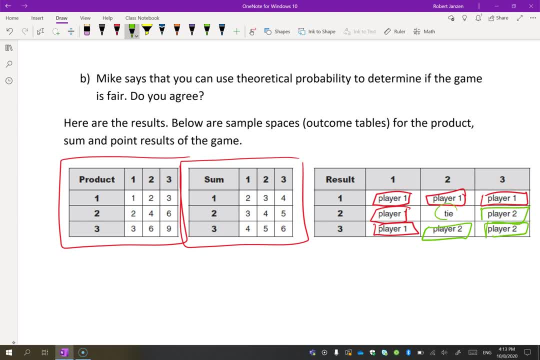 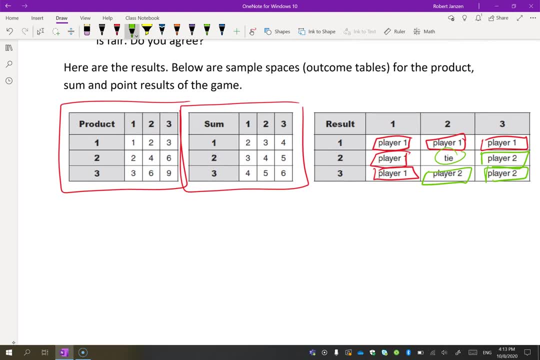 player two wins. And then there's the tie. So is this game fair? Well, you can see that player one has a better chance of winning Player one. so the probability of winning for player number one is five out of nine. For number two, the probability of winning is only three out of nine. 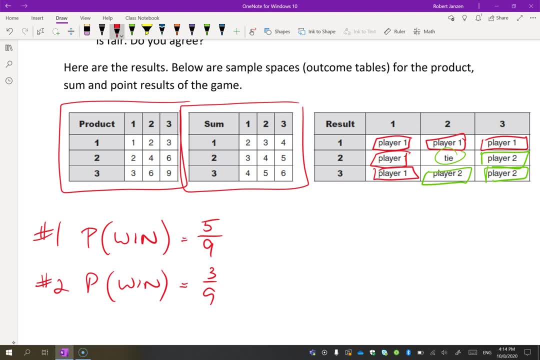 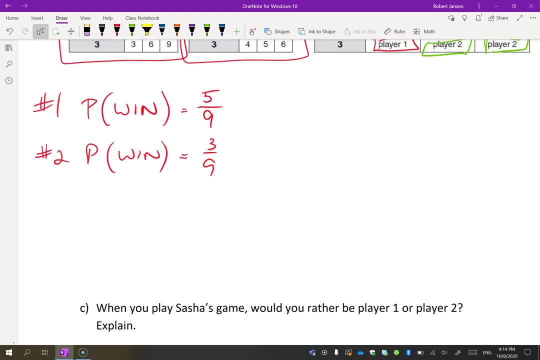 Okay, so that's how you determine if a game is fair. So question C is: when you play the game, would you rather be player one or player two? Well, assuming you want to win, you'd be player one. Okay, here's your homework for this lesson.